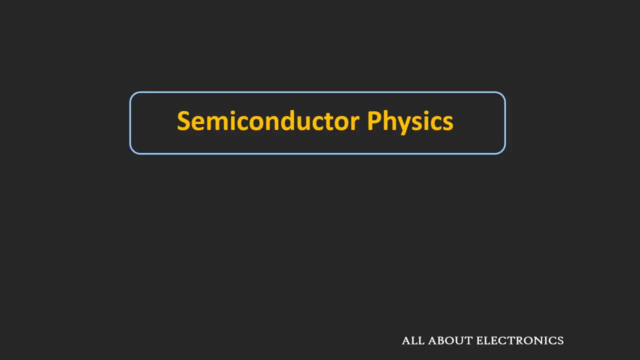 one needs to understand a little bit about the semiconductor physics and the semiconductor materials. So first of all, let us understand why the semiconductors are used in the electronics. And to understand that, first of all let us see the classification of the materials. 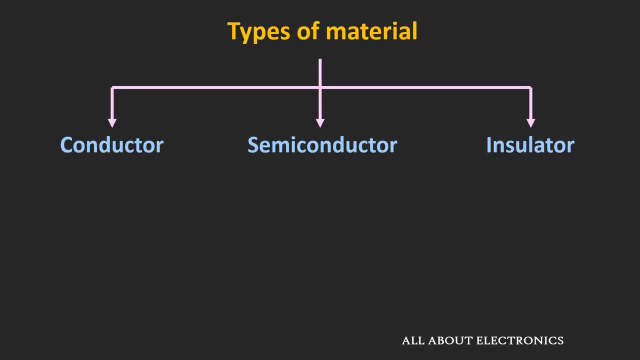 in terms of the conductivity. So, in terms of the conductivity, the materials are classified in three categories: Conductor, Insulator and the Semiconductor. Now, for any material, the conductivity defines how easily this material allows the flow of charge, And this conductivity is measured in Siemens per meter. 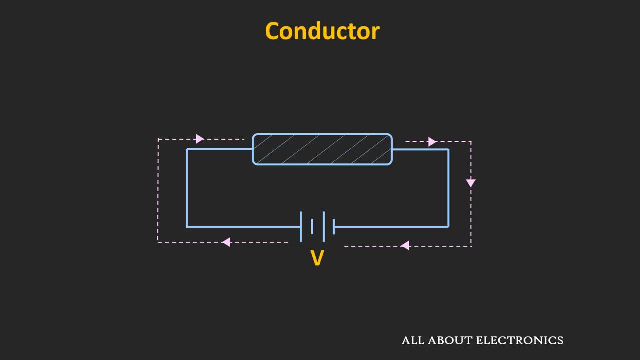 So the conductor has a very good conductivity. or we can say that whenever the voltage is applied to this conductor, then it allows the generous flow of charge. So the silver, copper, gold and aluminums are the few examples of the conductors. 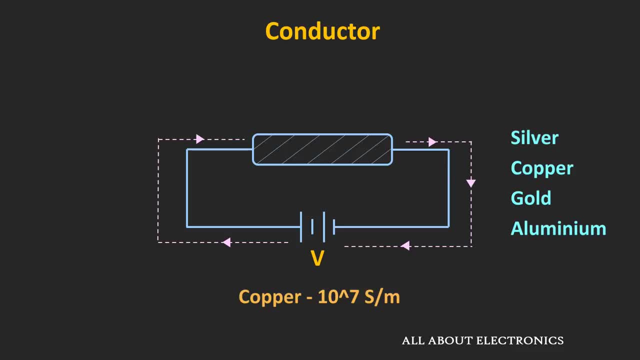 And if you take the example of a copper, then its conductivity is roughly around 10 to the power, 7 Siemens per meter. On the other hand, if you see an insulator, then it hardly allows any flow of charge, Or you can say that this insulator has a very poor conductivity. 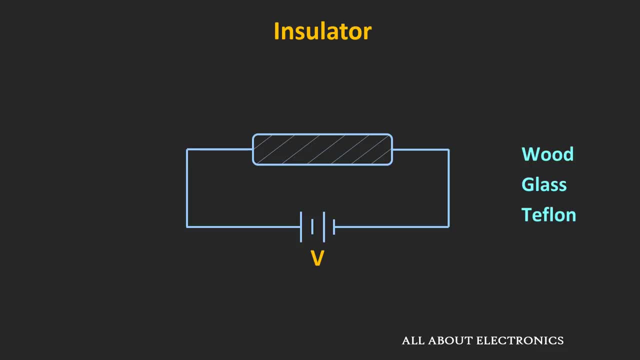 So the wood, glass, teflon are the few examples of the insulator. and if we take the example of dry wood then its conductivity is roughly around 10 to the power minus 14 Siemens per meter. So the two things are in here. 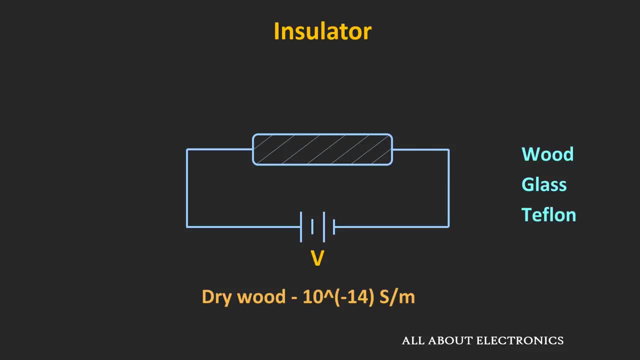 First of all just Sud etc. you just write add: if you come here and put compare, say this, inland terrain meter, so wood is a very good insulator. on the other hand, if we take the case of semiconductor, then its conductivity is between the insulator and the conductor. 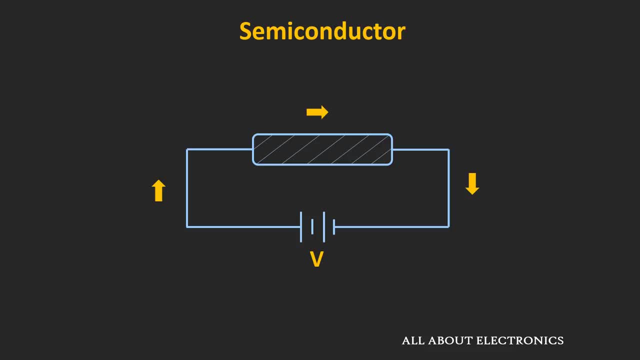 so whenever the voltage is applied to this semiconductor, then it allows the moderate amount of current and, moreover, that by adding the impurities the conductivity of the semiconductor material can be changed, and this property is very useful for designing the various electronic devices. so silicon, germanium and the gallium arsenide are the few examples of the 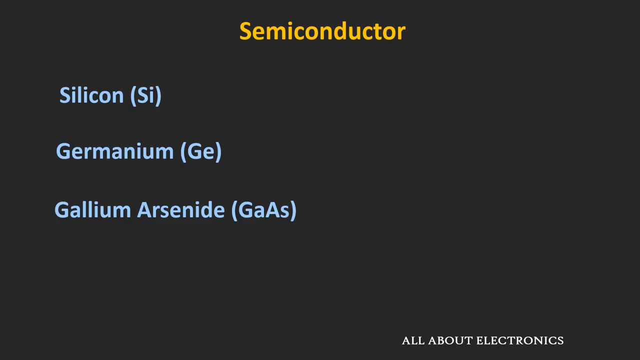 semiconductor materials. and here we will understand the behavior of the semiconductor by taking the example of a silicon which is extensively used in the electronic industry. now, the atomic number of the silicon is 14. so if we see the atomic structure of the silicon, it has 14 protons and the floating 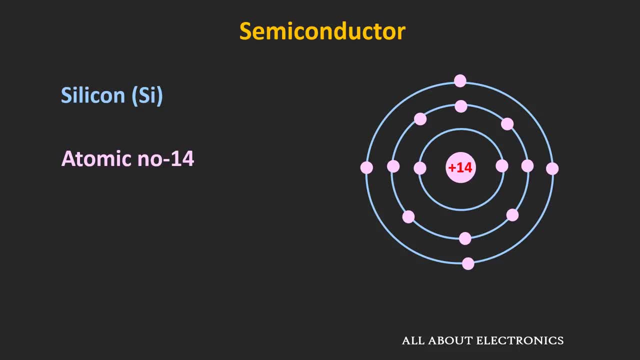 electrons. So these 14 protons resides in the nucleus and the 14 electrons rotates around this nucleus. And if you see the outermost orbit of the silicon, then it has a 4 electrons, or we can say that the silicon has a 4 valence electrons. 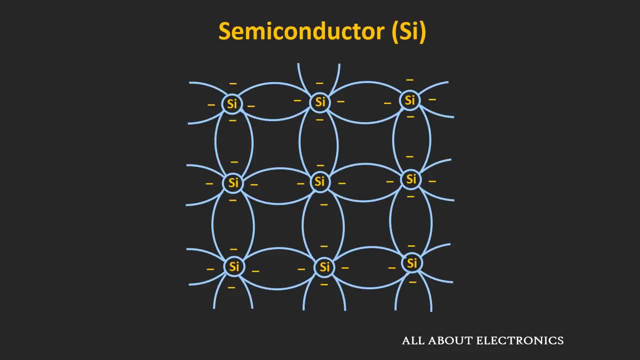 Now, whenever the silicon atoms combines to form a solid, then they arrange themselves in a particular pattern which is known as the crystal. And in this crystal structure each silicon atom shares its 4 electrons with the neighboring atoms, And the sharing of the electrons happens in a such a way that each silicon atom has 8. 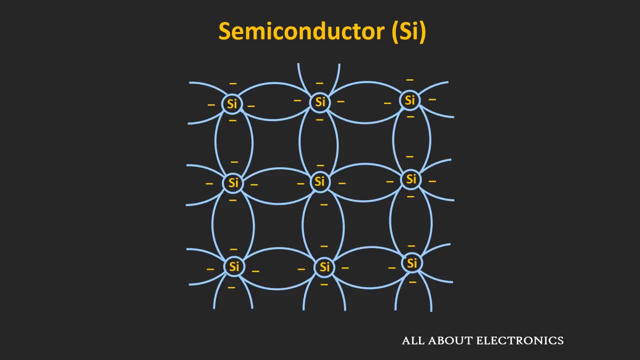 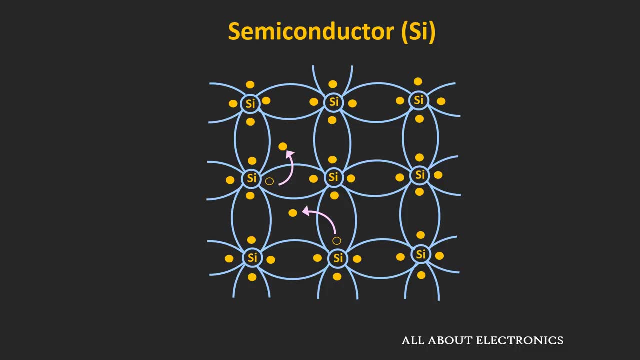 valence electrons And in this way, by sharing the electrons, this silicon atom forms the covalent bond. Now, at the temperature just above 0 degree Kelvin, due to the thermal energy, the atoms in the silicon crystal starts vibrating And due to this vibration, 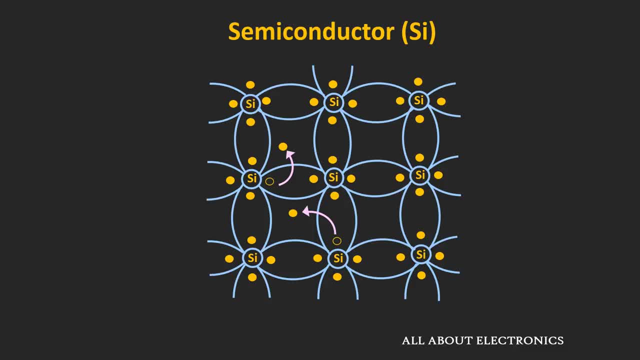 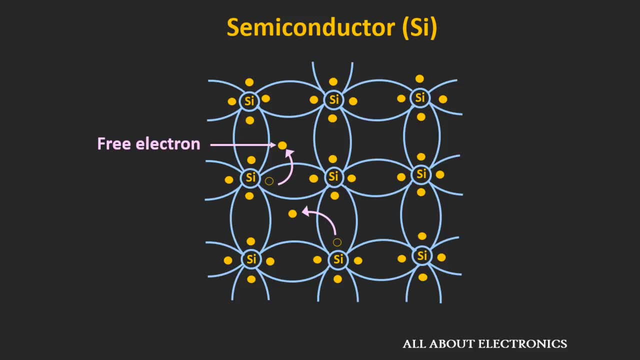 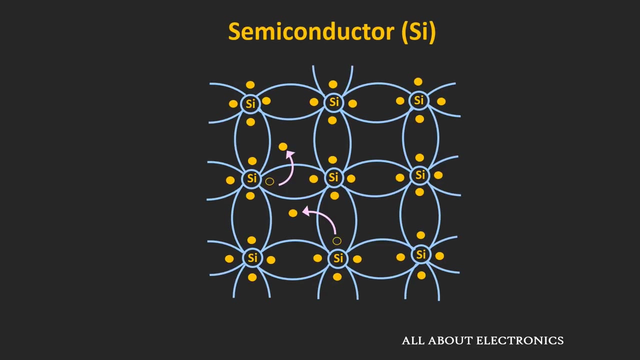 Some of the electrons may get enough energy so that they can break these covalent bonds, And while breaking these bonds, this electron will act as a free electron. So at room temperature you will find many such free electrons in this silicon structure. Now, whenever this electron departs from its position, then it creates a vacancy at that. 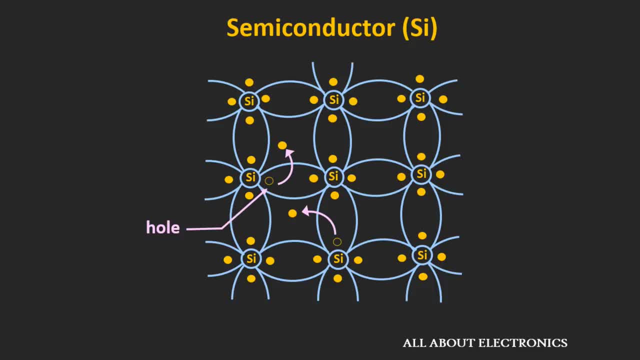 particular position, And this vacancy is known as the hole. Now we know that the charge of the electron is 1.6 x 10 to the power 2.. Now we know that the charge of the electron is 1.6 x 10 to the power 3.0.. 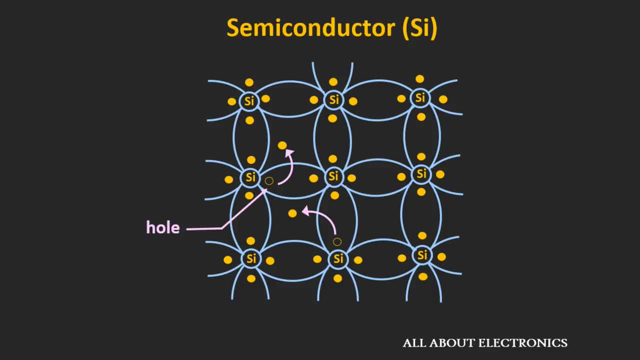 power minus 19 coulomb and it has a negative charge. So by not having an electron at particular position creates the positive charge and this positive charge is known as the hole. So this hole can attract the other free electrons which is roaming in the vicinity. So, as shown in the figure, let's say in this: 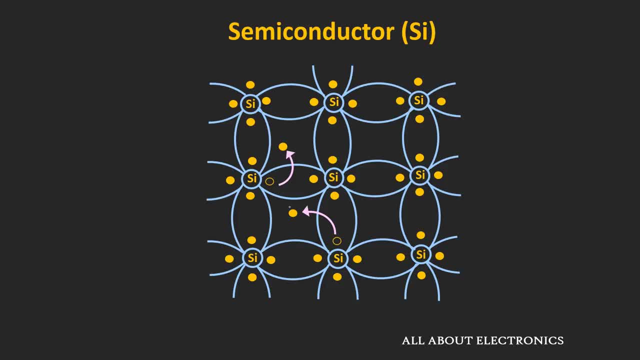 silicon structure. these two electrons are the free electrons and due to these two free electrons, these two holes has been created. Now let's say this electron gets recombined with this hole. So if it gets recombined with this hole, then the equivalent silicon structure will look like this. And here let's say, due to the 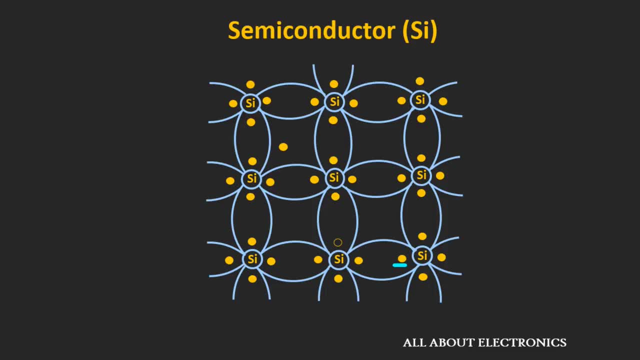 thermal energy, these electrons become free and it gets recombined with this hole. So in this way, for any silicon structure at room temperature the generation and the recombination of holes and electrons happens continuously. And one more thing: if you observe, for every generated electron the hole is also getting generated. So we can say: 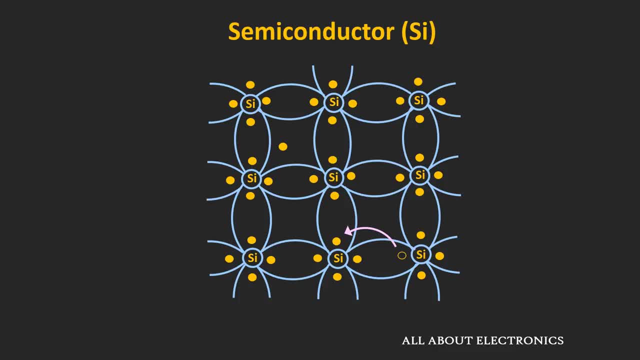 that at given temperature, the equal number of holes and electrons are created in this silicon structure. And one more thing: if you observe, as the electrons are moving from one place to the other place, the holes are also moving from one place to the other place. So in a semiconductor we get a flow of 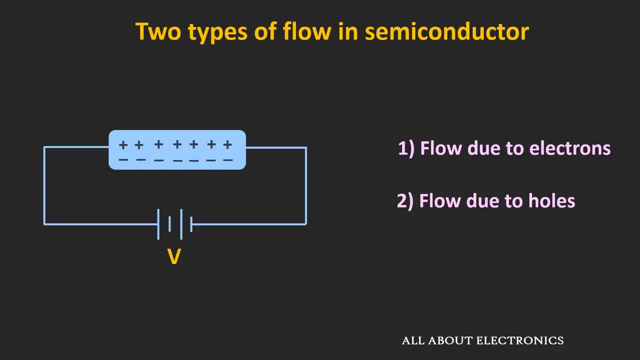 current due to the two types of charges: One is due to the electron and second is due to the holes. And this is the biggest difference between the conductor and the semiconductor, Because in a case of a conductor, we used to get a flow of current only due to electrons. Now this semiconductor can be classified in two. 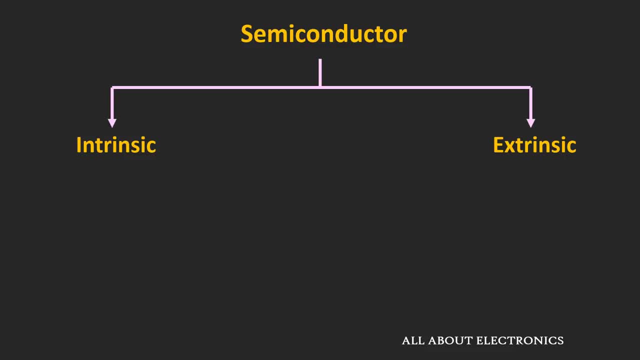 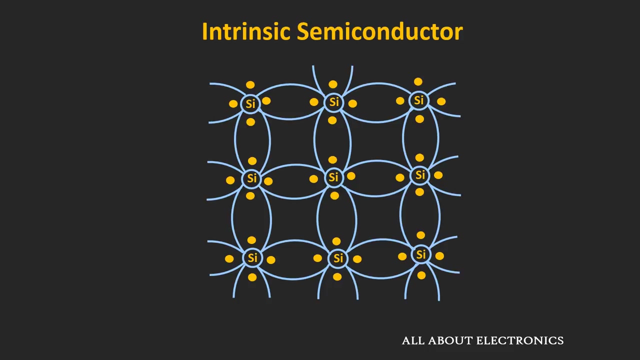 categories. One is an intrinsic semiconductor and the second is extrinsic semiconductor. So the intrinsic semiconductor is the pure semiconductor, without any kind of impurity atoms. So if we take the case of a silicon crystal, then in the intrinsic semiconductor all the atoms would be silicon atoms. On the 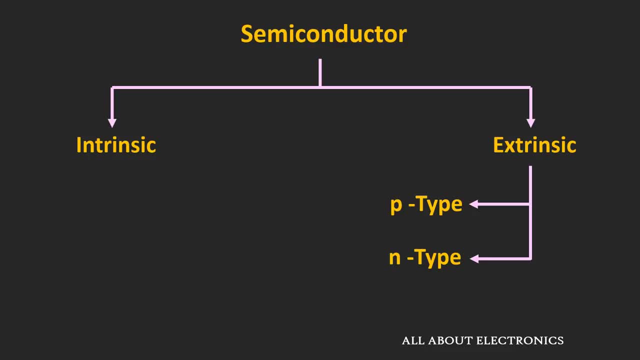 other end, in the extrinsic semiconductor, the external impurities are added to change the conductivity of this semiconductor And the process of adding these impurities is known as the doping. So by doping the semiconductor we can change the conductivity of the semiconductor material And by changing the conductivity we can control the semiconductor to behave in a 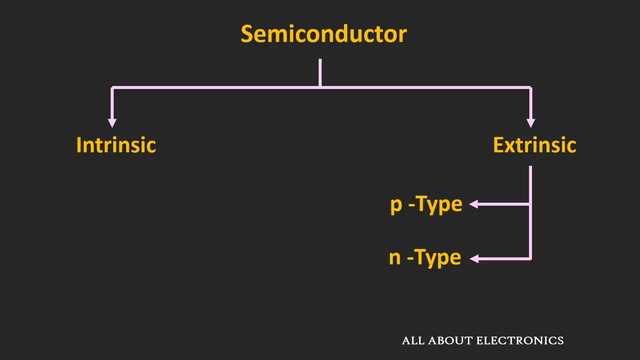 specific manner. So this is the reason these semiconductor materials are preferred in the electronic industry. So depending upon the type of impurity or the dopant, the extrinsic semiconductors can be further classified as a p-type or n-type semiconductors. So in case of a p-type semiconductor, the trivalent 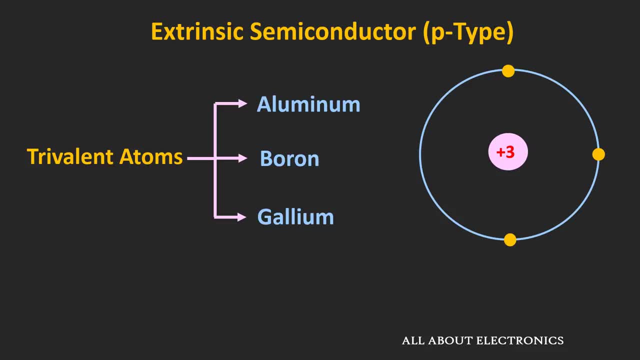 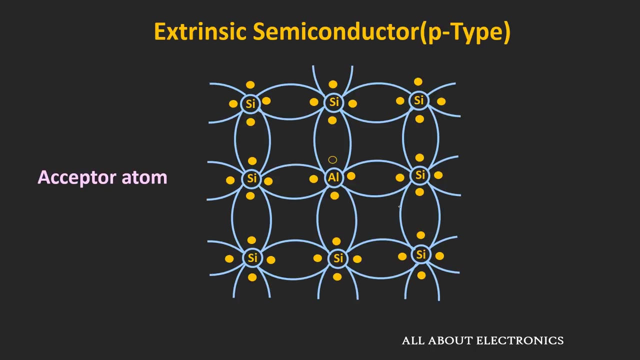 atoms are added with the silicon atoms. Now the trivalent atom means these atoms have three electrons in the outermost orbit, And the aluminum, boron and the galliums are the few examples of these trivalent atoms. So, since these trivalent atoms have three electrons in 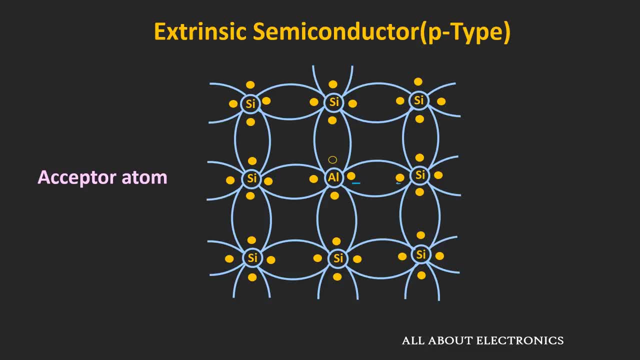 the outermost orbit. the three electrons are shared with the neighboring atoms But still, if you see, the one vacancy remains in the outermost orbit And due to this vacancy, we can say that the hole is created in the silicon structure. So we can say that every trivalent atom creates one. 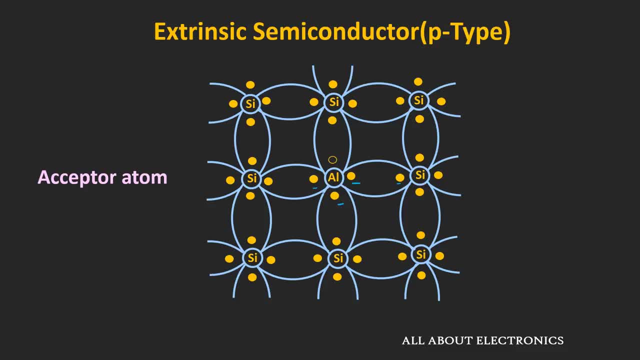 hole. So in this way, by adding the trivalent atoms, we can create excessive amount of holes in the crystal structure. And these trivalent atoms are known as the acceptor atom, because the each hole which is created by the atom can accept the external free electron. Similarly, by adding the pentavalent impurities, the n-type 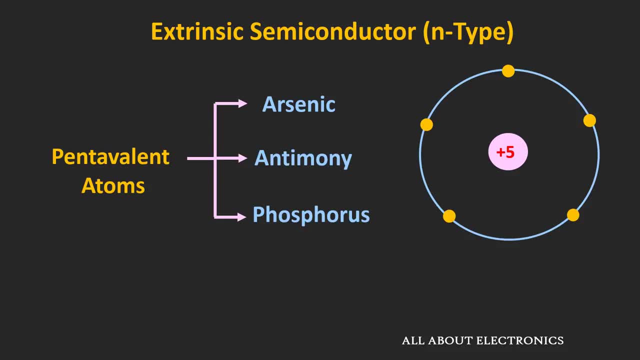 semiconductor can be formed. So in the pentavalent atoms there are five electrons in the outermost orbit And the few examples of the pentavalent atoms are arsenic, antimony and the phosphorus. So whenever the pentavalent atom is added, 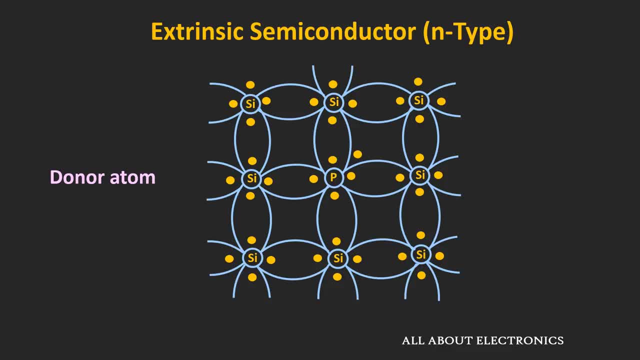 with the silicon atoms. then out of the five electrons, the four electrons of these pentavalent atoms will be get shared with the neighboring atoms, But still, if you see, the one electrons remains in the valence orbit. So this electron will act as a free electron and it can roam around in the crystal. 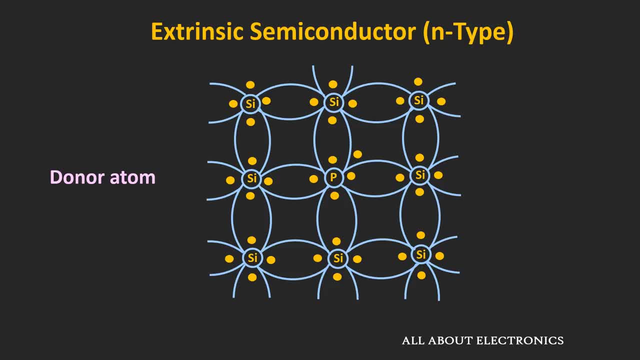 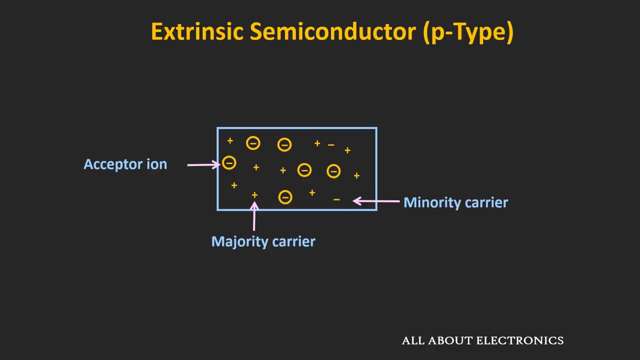 structure. So we can say that each pentavalent atom creates the one free electron. So by adding this pentavalent impurities we can create an excessive amount of electrons in the crystal structure. So in case of a p-type semiconductor there is an excessive amount of holes, While in case of n-type. 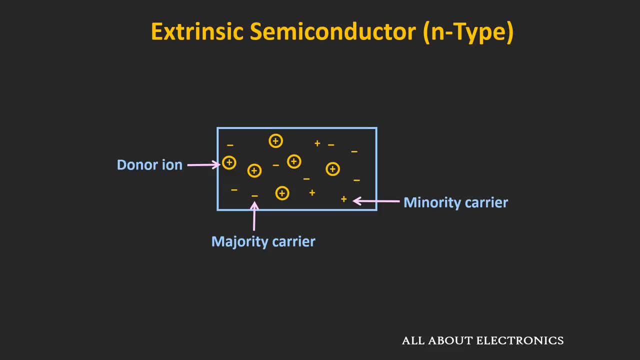 semiconductor there is an excessive amount of electrons. So in n-type, the electrons will be majority's carriers, while the holes will be the minority carriers. Similarly, in case of a p-type semiconductor, the holes will be the majority carrier and the electrons will be the minority carrier, Meaning that whenever we apply, 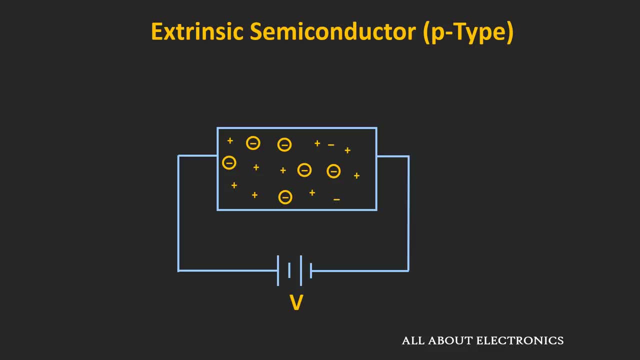 the voltage to this p-type semiconductor, then the majority of the current which we will get is because of the holes. So whenever we apply a voltage source to this p-type semiconductor, then the holes will get activated towards negative terminal, while the electrons will get attracted towards the positive terminal.